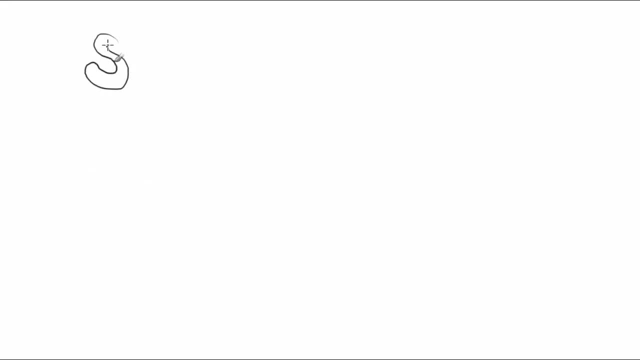 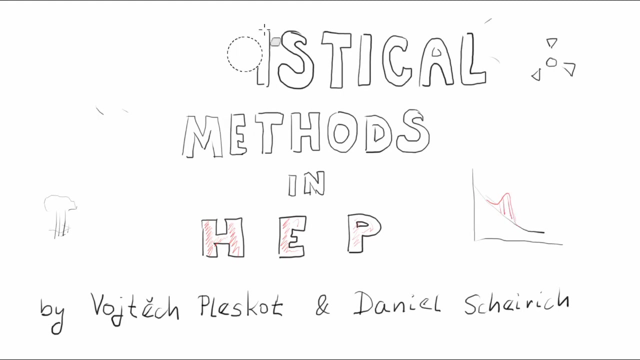 then let me assure you that, yes, this is the channel on statistical methods in high-energy physics and we are going to talk about limits, on parameters of new physics theories. Let's imagine we've done our experiment and we didn't find the signal we were looking for. 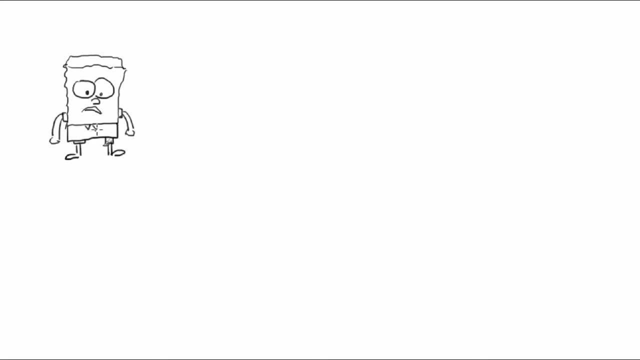 A hypothetical particle, the Spongebob boson, let's say. However, we shouldn't have any bad feelings about the cheerless result of our experiment. We cannot order nature that this and this particle must exist. We should definitely report the result of the experiment to tell people that the particle doesn't exist. 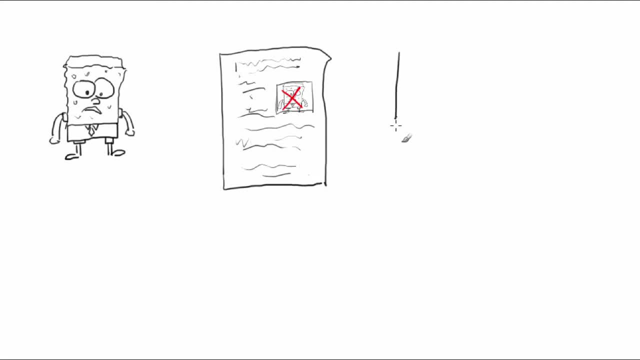 Almost always new theories have three parameters and we should work hard and exclude the biggest possible part of the parameter space. Typical parameters are masses of new particles, coupling constants or just branching ratios, cross-sections and so on. A hypothesis about a new theory is determined by fixing values of all three parameters. People set limits on the three parameters. 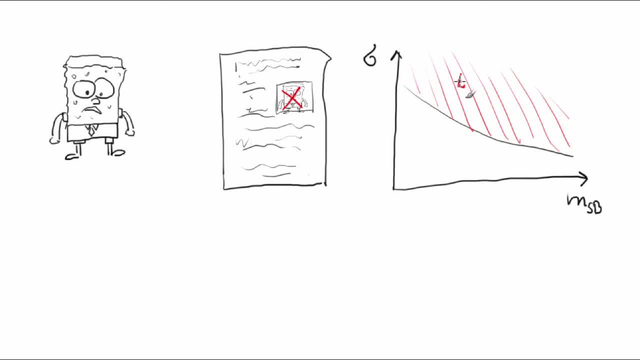 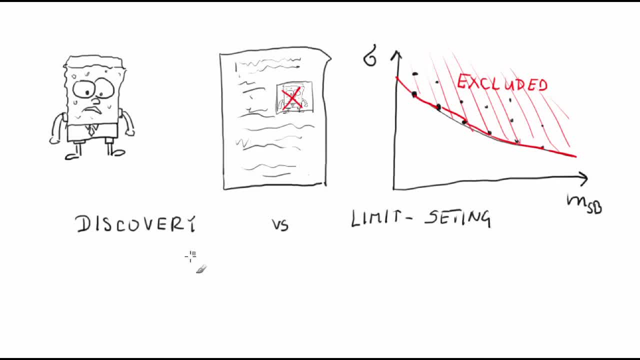 The size of the test. A discovery in particle physics has most often very far-reaching consequences. Therefore, people want to be extremely sure about the size of the test. Therefore, people want to be extremely sure about the size of the test. 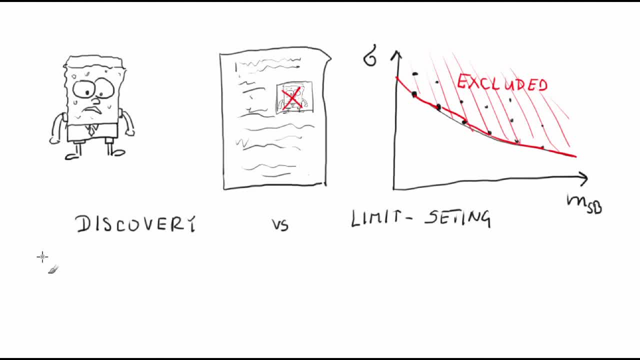 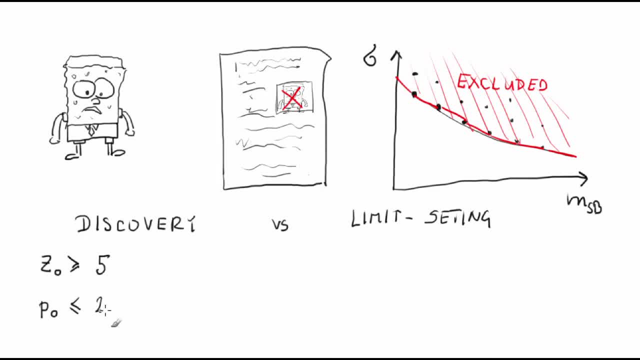 This corresponds to a probability of 2.9 times 10 to the minus 7.. On the other hand, an exclusion of one point in a huge parameter space of one of many new theories has less consequences and therefore a typical size of a test is much lower. 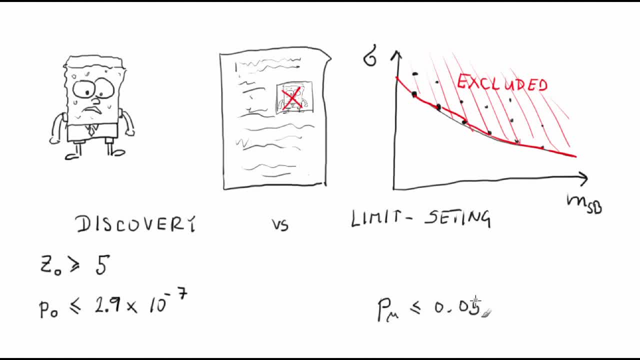 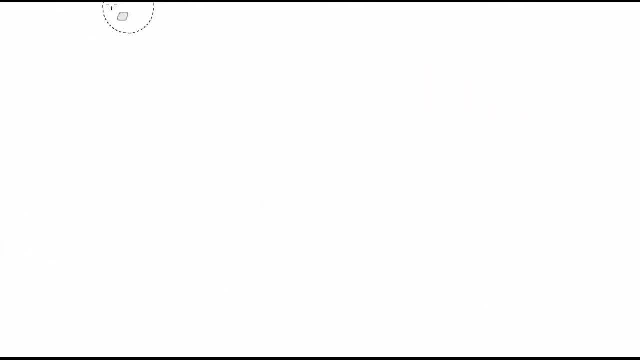 The most common test size is 10 to the minus 7.. This is now 0.050. in the previous example In one of the previous videos, we defined the test statistic T sub mu vector. T sub mu vector is equal to the pencil index square minus 2. log L of mu vector. 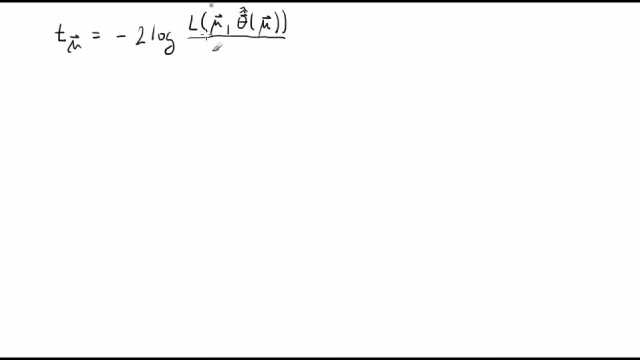 theta vector head-head of mu vector over L of mu vector head. theta vector head. This is a one tooth flat. We also said that this test statistic wasn't suitable for discoveries because of reporting discrepancy with the background-only hypothesis for both excesses and deficits of data events. 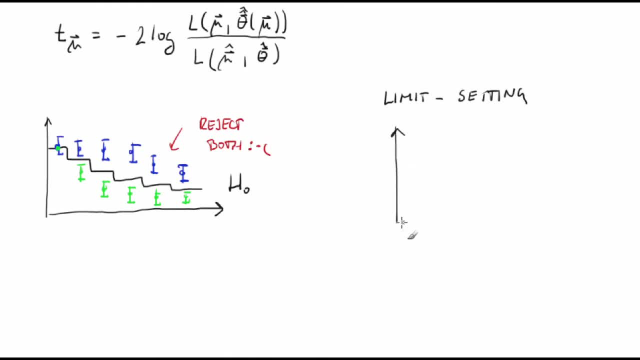 For the same reason it is not suitable for limit setting, neither An obvious remark When setting limits. the null hypothesis H0 that we test is the new theory, And all its three parameters are fixed to some values. The alternative hypothesis predicts just background. 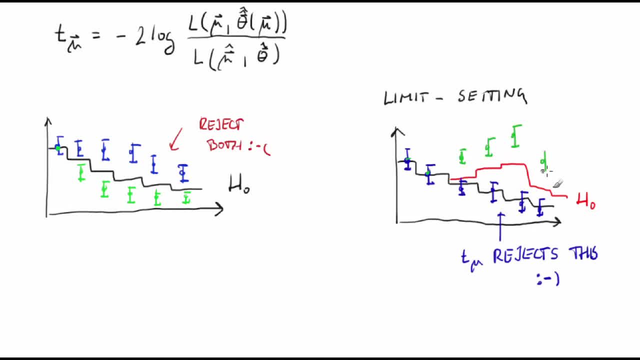 Definitely we don't want to exclude a theory if we observe an excess of events over the background-only expectation. In analogy with the test statistic for discovery, let's define the one-sided test statistic for exclusion: Q sub mu Is equal to T sub mu if mu hat is lower than mu. 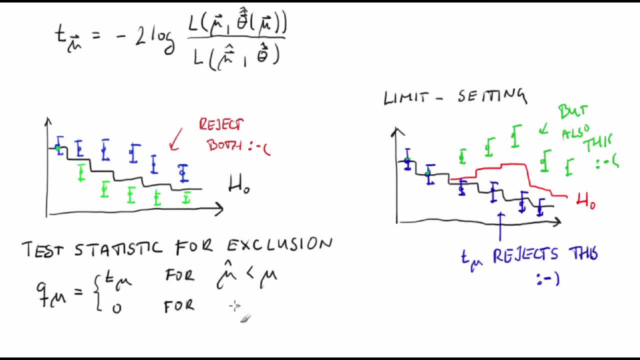 And it is equal to zero if mu hat is greater than mu. Thanks to Mr Wilkes and his theorem, we know the distribution of this test statistic in the large sample limit. Large sample means that there are at least about five events in each bin of our sample. 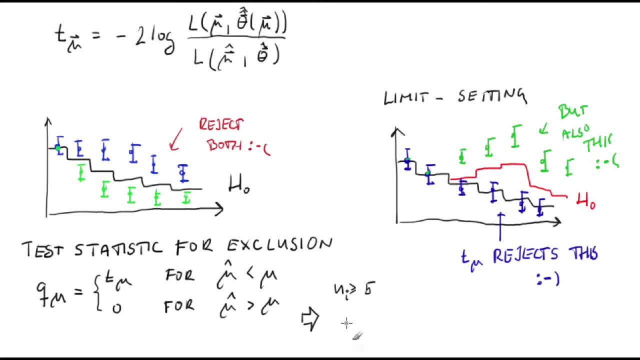 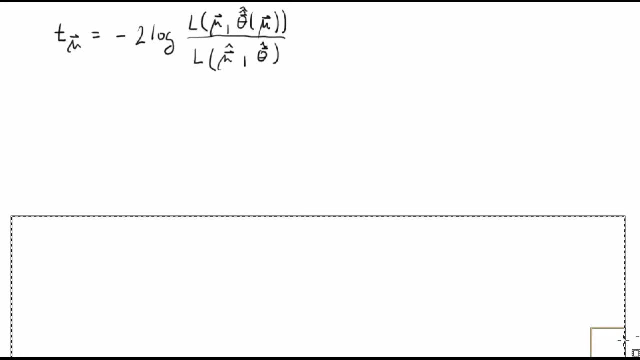 Now the distribution F of Q sub mu, given mu, is approximately equal to one-half of the delta function of Q sub mu plus one-half of the chi-square distribution. with one degree of freedom of Q sub mu, Then formulae for the p-value and significance are: 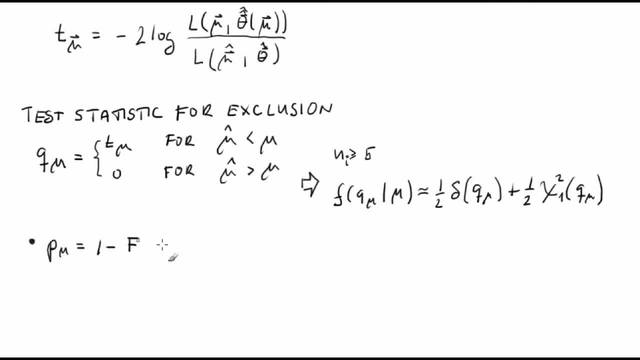 P sub mu is equal to one minus the cumulative distribution of Q sub mu given mu. And this is approximately equal to one minus the cumulative distribution of the standard Gaussian phi of the square root of Q sub mu. Z sub mu is equal to the inverse of phi of one minus P sub mu. 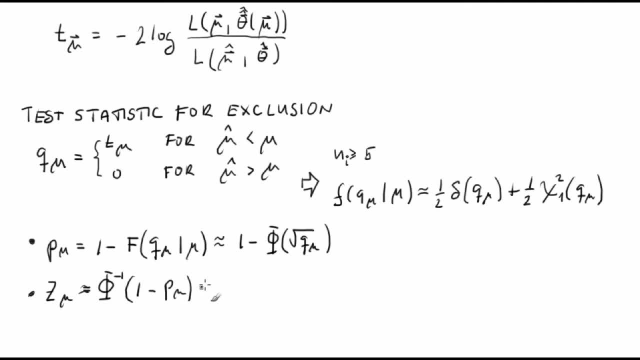 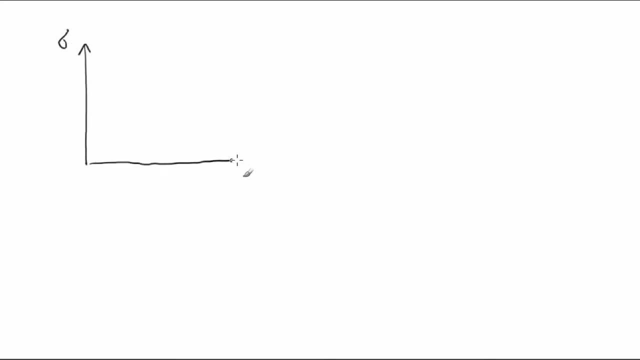 And this is approximately equal to the square root of Q sub mu. A very common money plot is the cross-section upper limit as a function of one chosen parameter of the new theory. All other theory parameters are fixed to some representative values To make the plot. 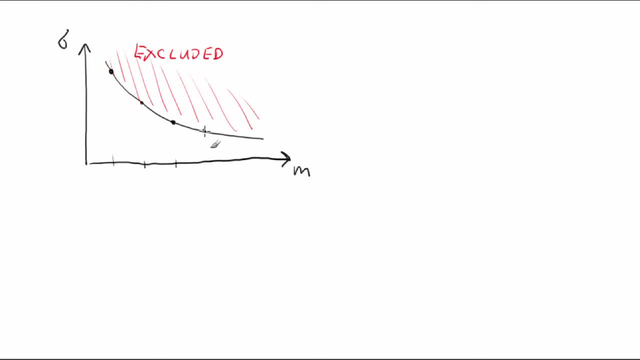 we first define a grid or a step size in the one-dimensional parameter space. Then, for each point we solve the equation: P sub mu is equal to alpha. In practice, we perform a set of tests where each test focuses on a different value of mu. 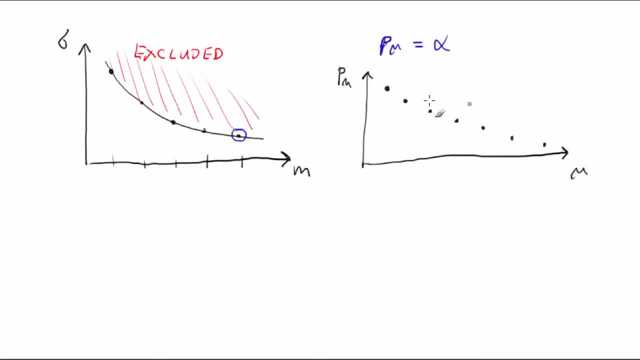 We can plot the dependence of the p-value on mu. The interpolation between adjacent points can be just linear. The mu-value that yields the p-value equal to alpha is our upper limit on mu. The upper limit on the cross-section is a product of the nominal cross-section. 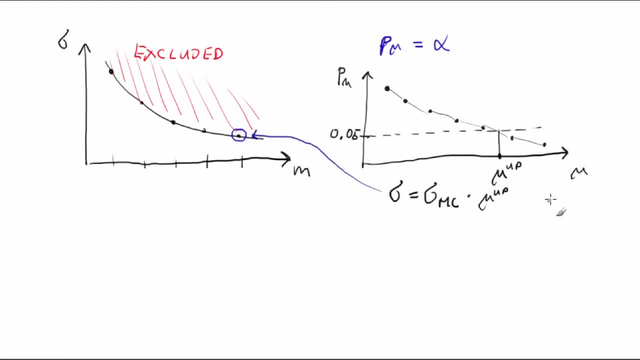 and the upper limit on mu. Up to now, we talked about observed limits, those based on real data. However, people are also curious about expected limits, Hypothetical limits we could get in case of no-signal observation, The median of the p-value. 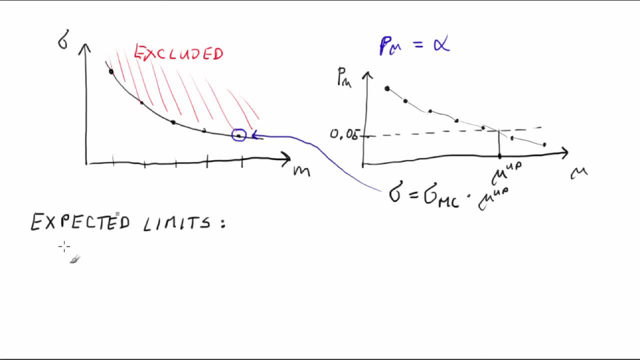 if no signal exists, can be estimated very accurately with the use of the Asimov dataset. When setting limits, the Asimov dataset is equal to the background prediction. For example, the expected upper limit on the signal strength is determined by solving. 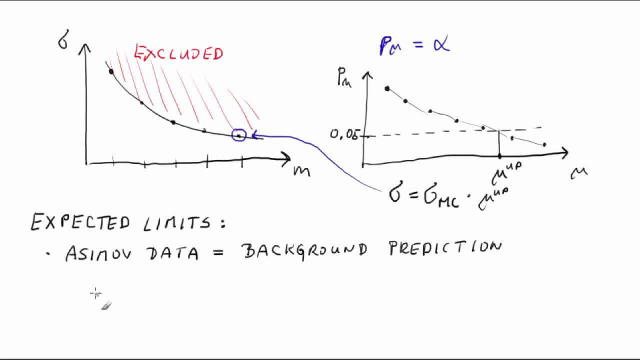 the following equation: for mu, Median of p-sub-mu, given the hypothesis of mu equal to zero, is approximately equal to one minus phi of the square root of q-sub-mu A, and this is equal to 0.05.. When setting limits, 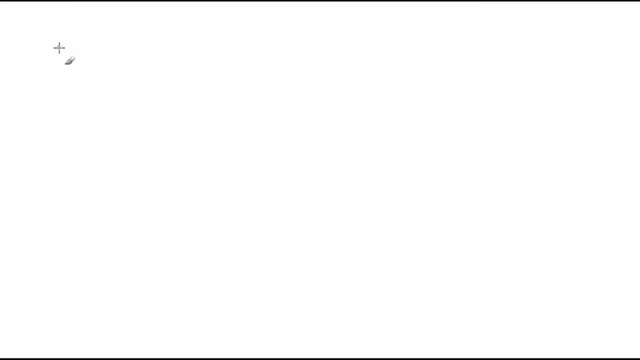 we can easily run into a situation in which the null and the alternative hypotheses predict a very similar distribution of the test statistic. Obviously, such a test has a very low power. In an extreme, but not uncommon case, the power can be as low as alpha. 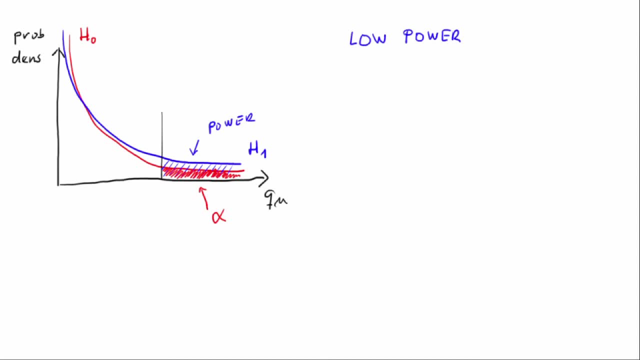 If this happens, and assuming the background-only hypothesis is true, there is a probability of alpha or similar to reject the new physics model in a test that is insensitive to it. Unfortunately, we drift towards this regime when calculating upper limits on mu. We test lower and lower values of mu. 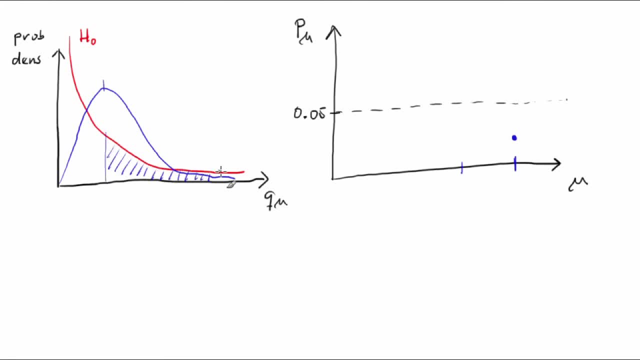 until we find such mu for which p-sub-mu is equal to alpha. Also note that we should get negative upper limit on mu in fraction alpha of k-sub-mu. This is a very common hypothesis Whenever q-sub-mu picked from f of q-sub-mu given 0,. 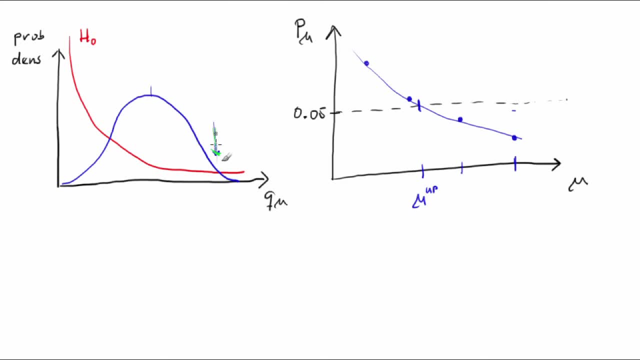 is in the high tail of this distribution tail that has an integral of alpha. the curve for p-value, as a function of mu, doesn't cross the line at alpha for any positive mu value. A solution to this problem is to replace the p-value. 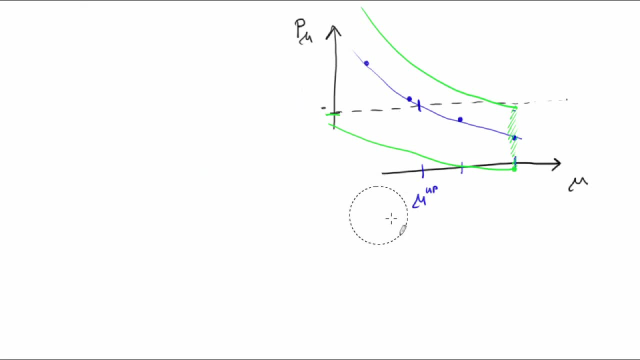 with some quantity that takes into account the power of the test. Such a quantity can be: cl-mu is definitorically equal to p-sub-mu over alpha. Here, 1-p0 is equal to the integral from q-sub-mu ops to infinity.